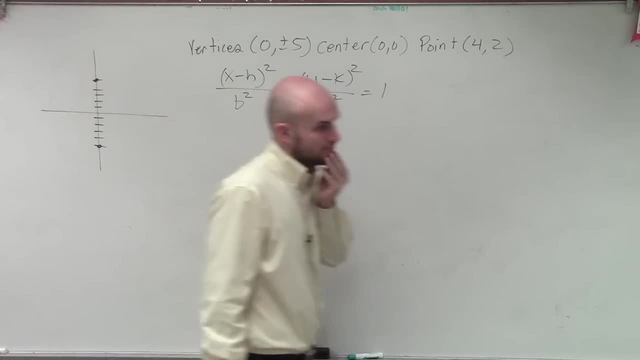 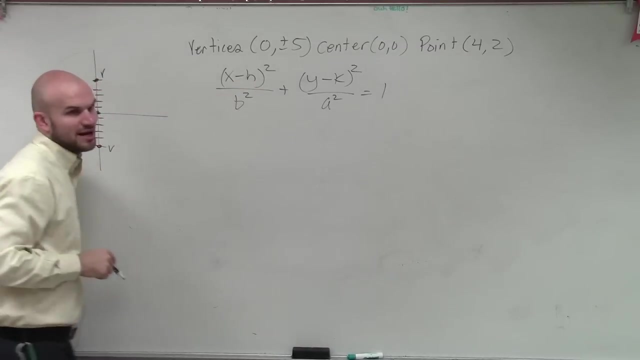 It's horizontal, the a will go under your x. Okay, All right. So we know here's our two vertices, and that's all we got. Now we also know the center's at zero, zero, right. So, ladies and gentlemen, do I really even need my h, my k right now? They're zero, zero. 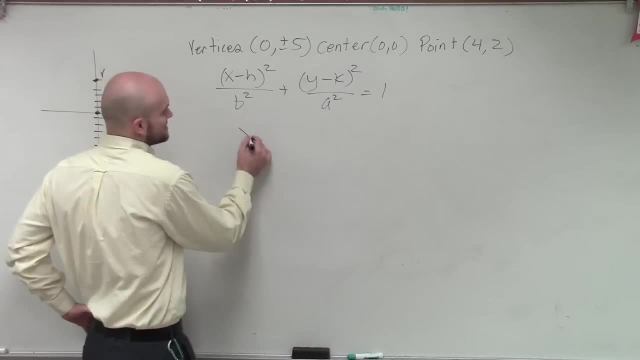 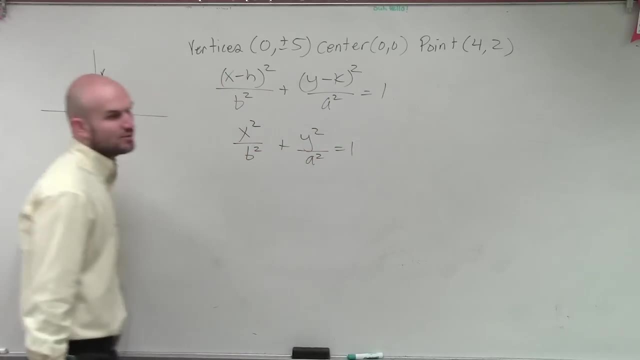 right, X minus zero is just x. So I'm going to simplify this equation just to x squared over b squared, plus y squared over a squared, And then I'm just going to find out that this is a vertical and this is a horizontal. 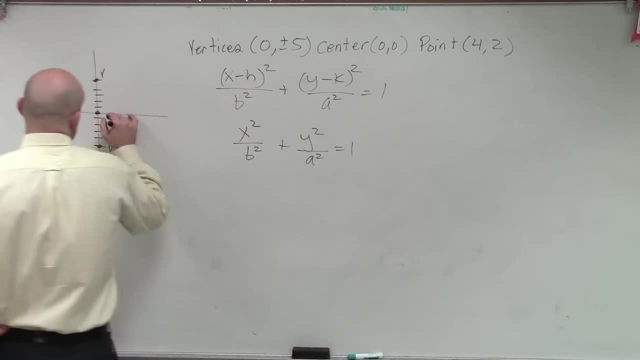 vertical, This is a vertical and this is a horizontal. All right, what I do is I get this entire thing here, What I call a spot-sqrt. Let's call this a spot-sqrt, Let's call it a point-sqrt, So we'd get 2.這麼. what does that do? Well, it adds up. 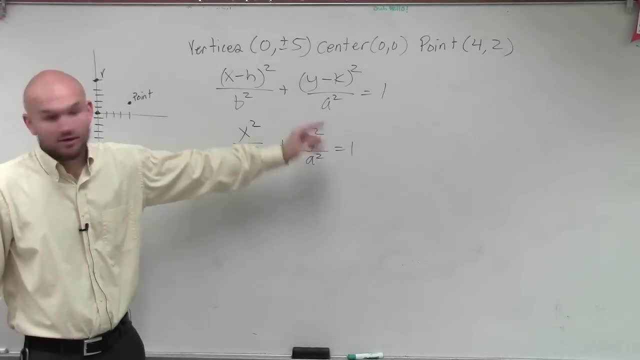 We actually divide that by two, ит adds. we added up the upper, it adds up the lower. divided into two, It makes all right. so we add that up. whatever this length has to do with the distance. Wait a minute. Yep, For x squared over b squared over b squared over a squared. 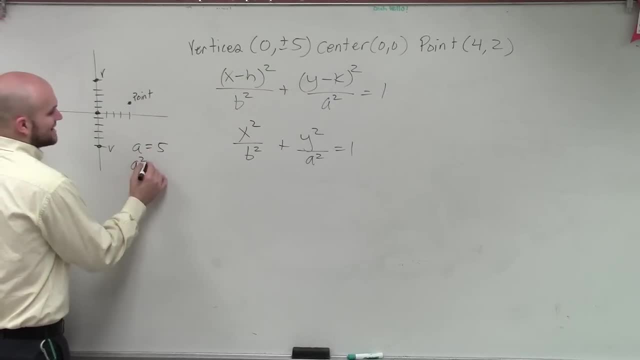 my end Vlog was 3: か45'sqrt. All right, Remember a trajectory美味 Makes this equation a. So if a equals 5, then we can say a squared equals 25.. So let's rewrite that. But our problem is we don't know what b is. 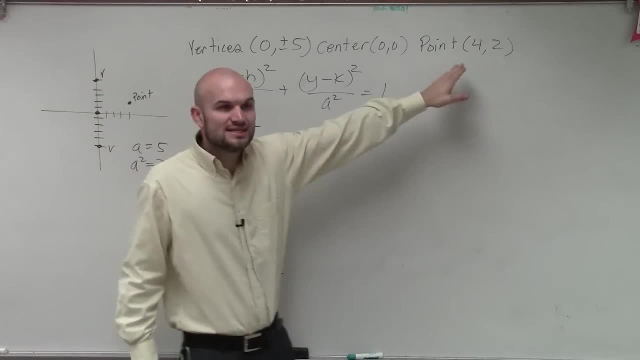 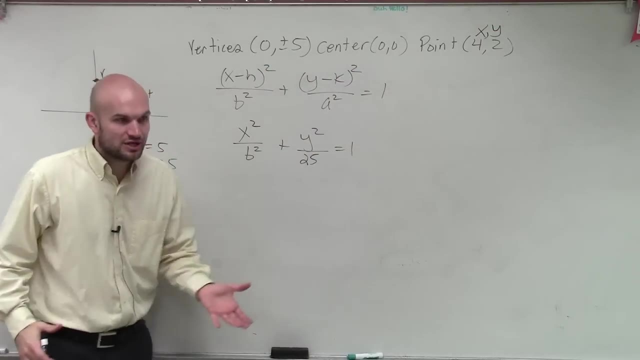 or we don't know what the distance to the foci is, But we do know what a point is. we do know a point- 4, 2, which remember, ladies and gentlemen, when you're dealing with an equation and your x and y coordinates represent all the possible points. 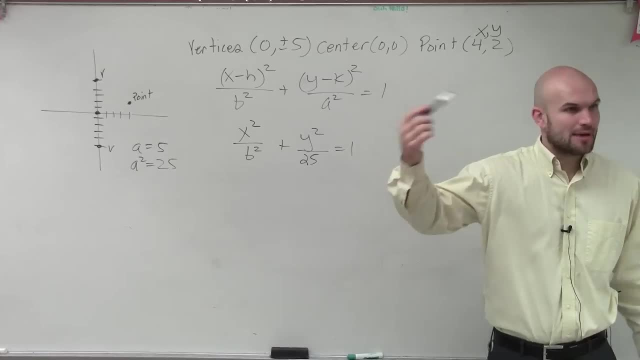 on your graph Because remember, for this ellipse, how many points are there on an ellipse? 1, 10,, 20, 30?? There's infinite many. right, And remember, x and y represent all of those points. 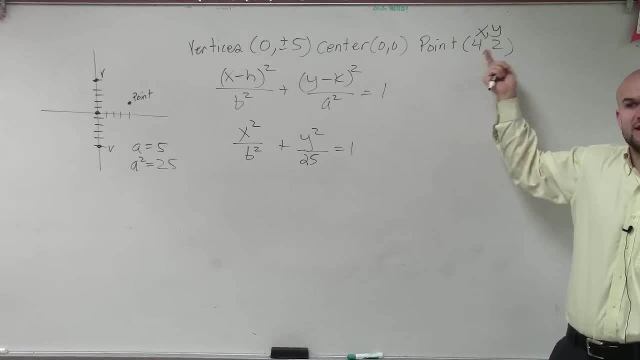 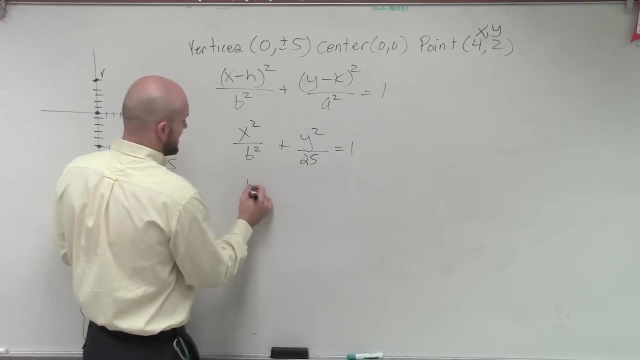 But if they give you one point that's on the ellipse, we can use that to help us find our other values. So what we're going to use is we're going to say, alright, 4 is going to be x squared. 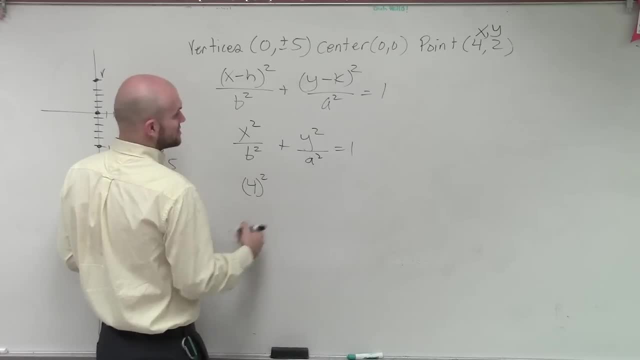 Actually I'll just keep that up. I'll put it in a second. So we'll say: 4 equals x squared divided by b squared, which we do not know, plus y squared, which we'll say is 2,. 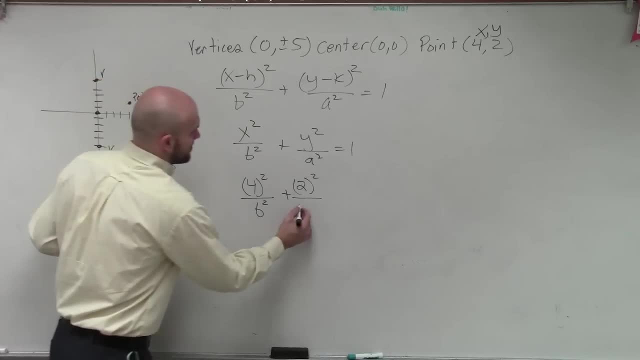 and then we said a squared, which is 25, equals 1.. Now we've got to do a little mathematics: 16 over b squared equals 4,, I'm sorry, plus 4 over 25 equals 1.. Well, guys, going back to algebra, 1,. 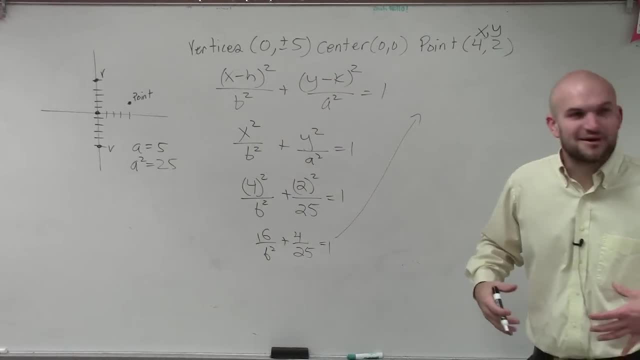 I know you're going to get you automatically get like the sickness You see. oh no, I have fractions and I have to add, subtract and do all that kind of stuff, But that's all we're going to do, ladies and gentlemen. 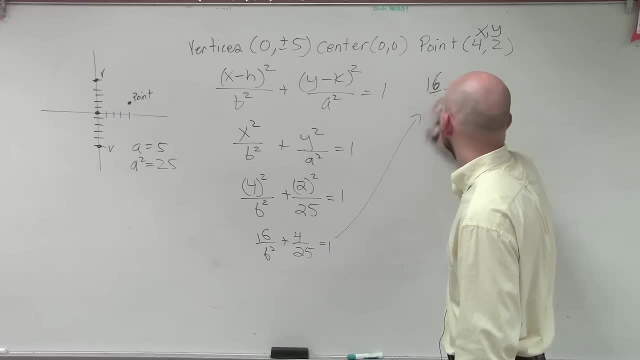 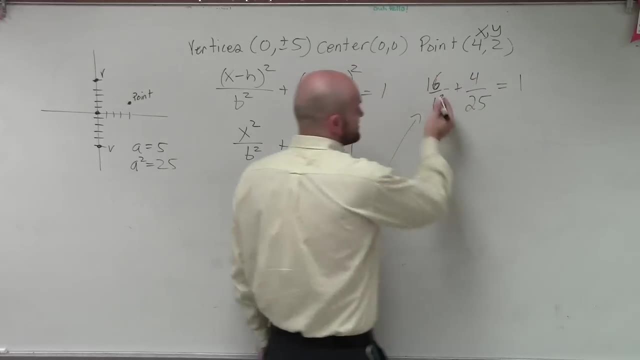 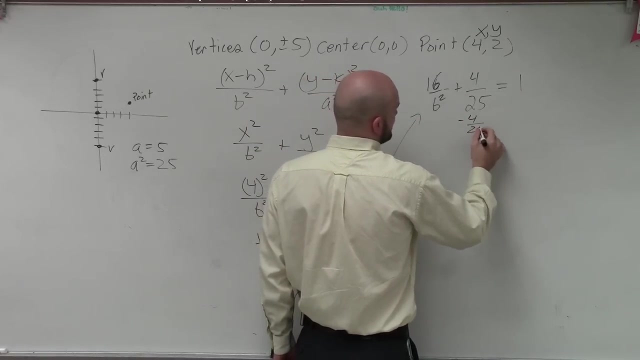 is just go back to. I promise it won't be that bad. So now to solve for b squared, I'll subtract minus 4 over 25.. Can I like cross multiply? You can't cross multiply them until you have a proportion. 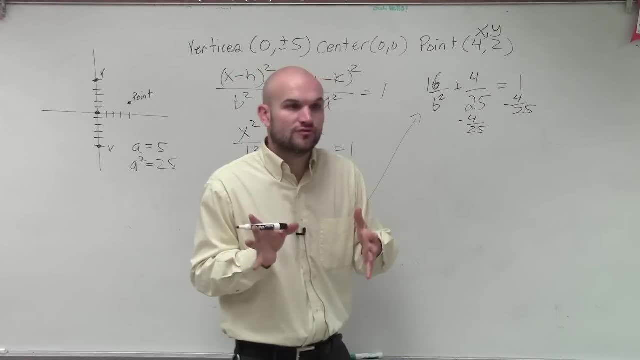 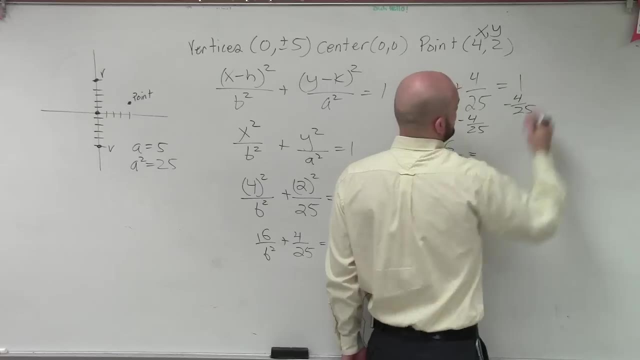 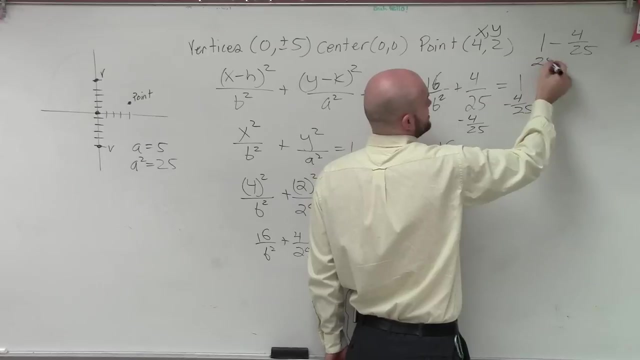 which we'll do next, which means we're going to have a fraction equal to another fraction. So now I have 16 over b squared equals. well, what's? 1 minus 21 over 25.. Right Well, 1 minus 4 over 25,. 1 rewrites to 25 over 25,. 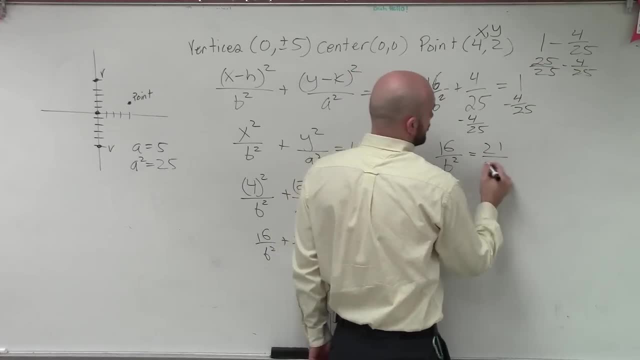 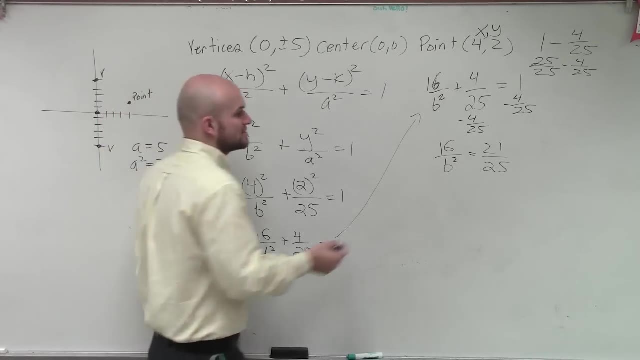 minus 4 over 25, which, yes, is 21 over 25.. All right, So now we have 16 over b. squared equals. well, what's 1 minus 25.. Now you have a proportion. so now, if you want to solve, 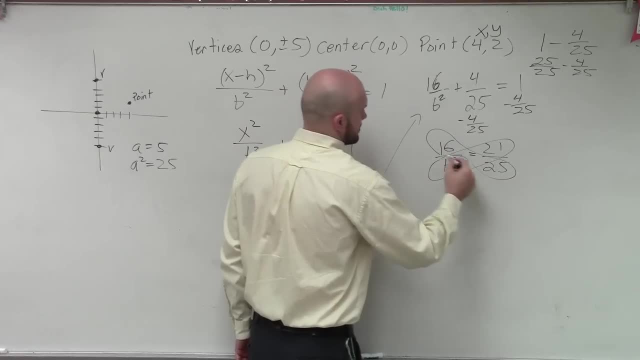 by cross multiplication. you can. There's other ways to do it. So you can do: 16 times 25 equals b squared times 21.. Now I don't have my calculator with me. 400 equals- This is what 400.. 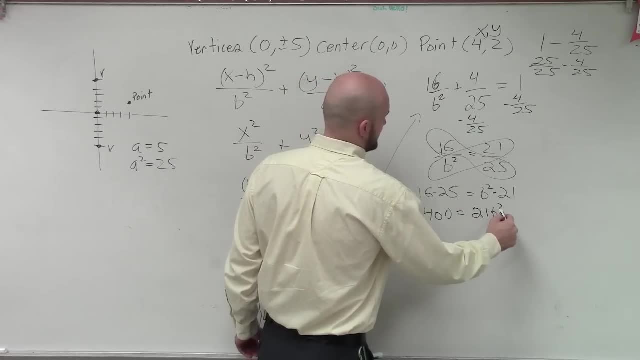 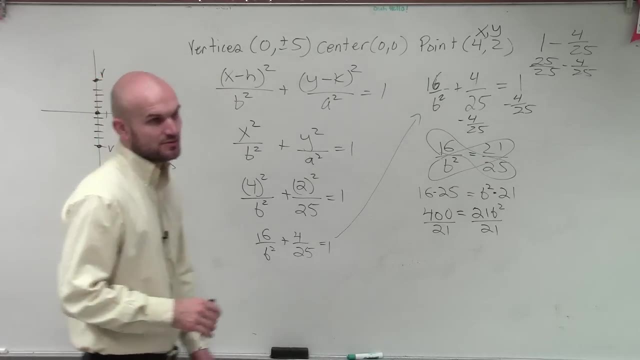 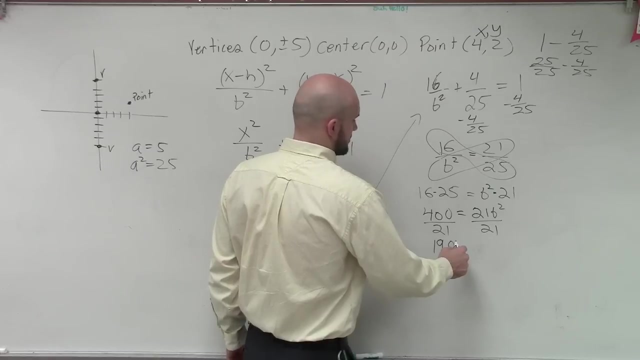 Equals 21 b squared, And then you divide by 21.. Oh wait, is that a 216?? No, it's 21 times b squared, Equals 19.0476.. Zero what? 7, 6.. 476.. 4, 7, 6.. 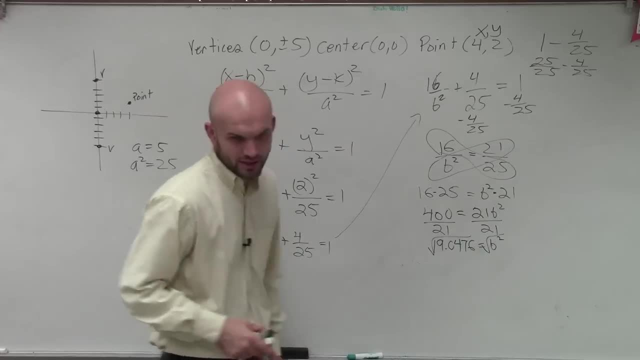 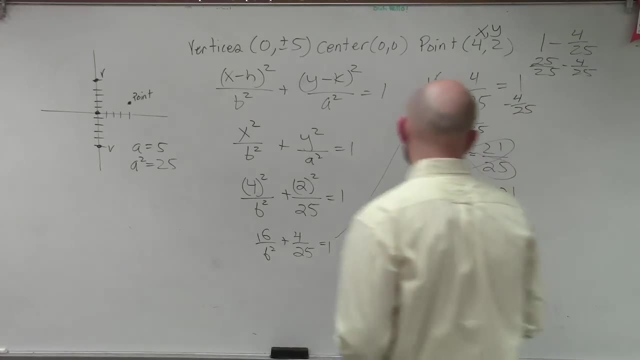 And then square root. You check my notes with this, and then you take the square root and what do you get? Oh wait, you don't need a b squared right, We don't need it, We just need b squared right. 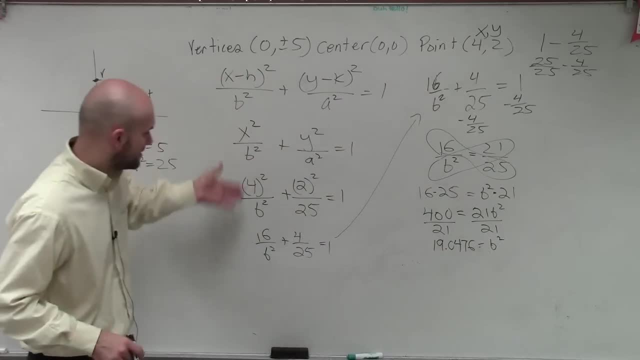 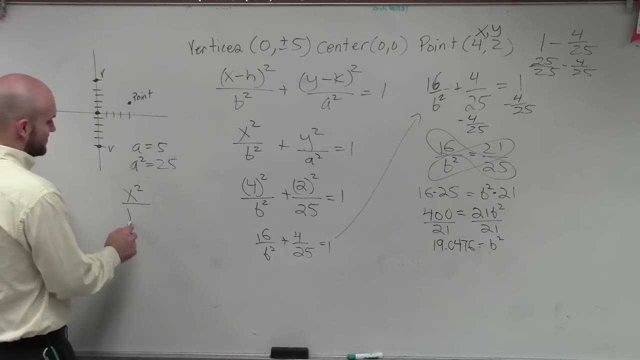 We don't need a b, Sorry, We just need the b squared. So now, if we have x squared over, since it's horizontal, we can say 19,, which I'll just round it to our actually 0.05 equals- why am I saying equals plus y squared over a. 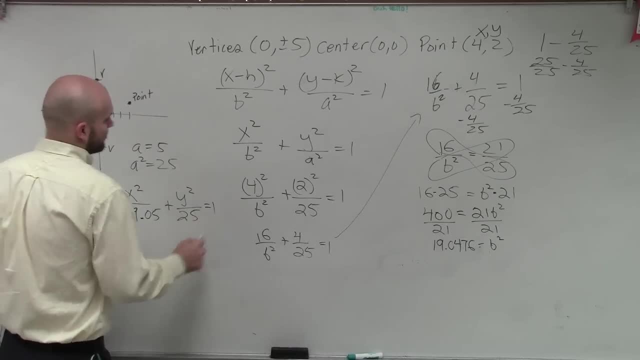 squared, which is 25.5.. That's right, 25 equals 1.. So let me just double check my work to make sure I had everything correct. I figured we probably made a mistake, so let's go and take a look. 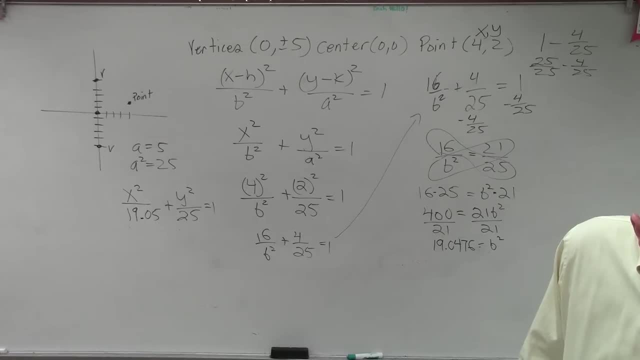 Well, wouldn't you? I think the book, I think half the note would be wrong. Let me see what my The book says. like 400 in it. I didn't know that was an open book. Wow, That's just. 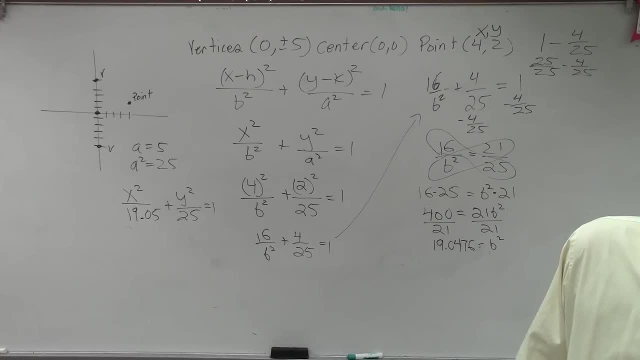 Why is it a waste? It was wrong. Why is it a waste? It was wrong? Okay, Well, there is a mistake in there somewhere, so it doesn't mean the whole problem is like a waste. What problem is this? 23.. 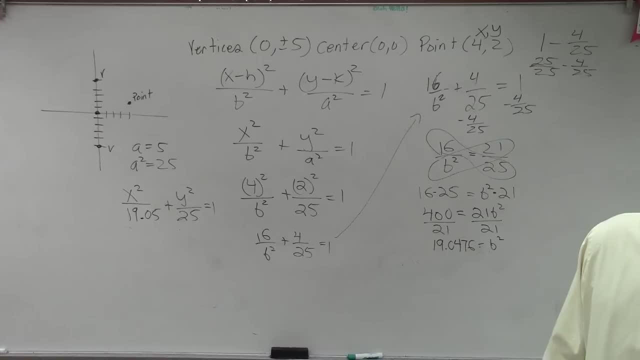 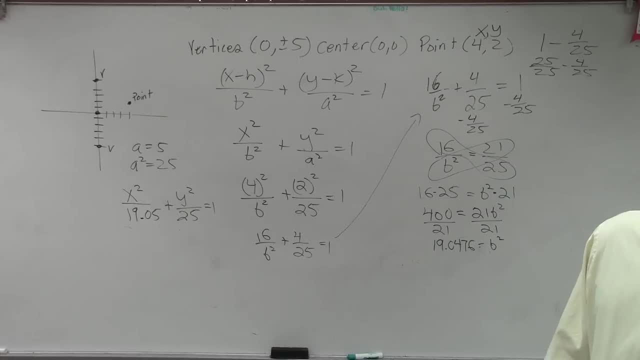 I don't know 23.. 23. Sorry, Okay, I was going to say: What's 400 divided by 21?? That was the ninth. It's right there. They just left it in fractional form, That's it. 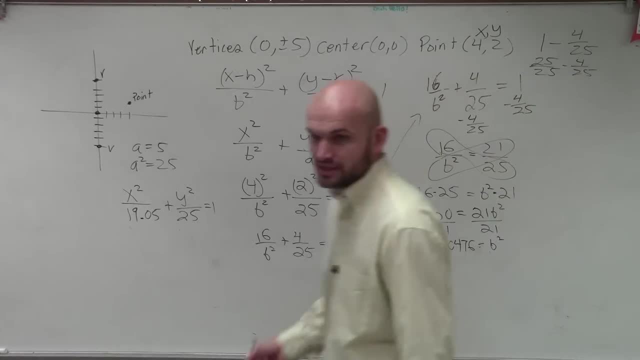 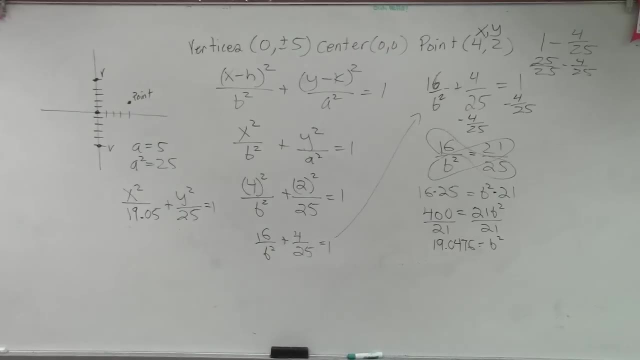 That's theıs, Thank you.